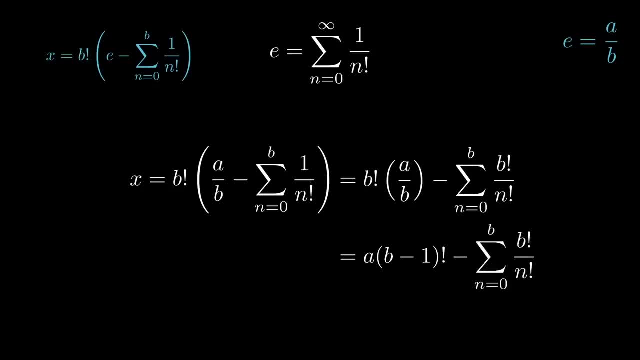 What should we notice here? Well, remember, b is a positive integer itself, so this first quantity is going to be an integer and this sum is going to be an integer as well. That's because b is going to be greater than or equal to n, for all n in this sum. What's the consequence of this? 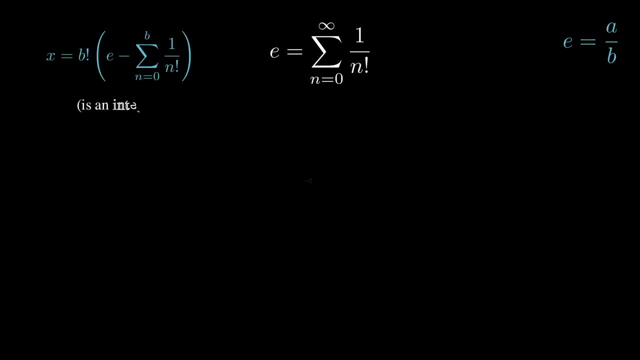 x is an integer, x is an integer minus an integer, or x is an integer. Let's substitute our other representation for e into x, this infinite sum. Both of these are really summing the same thing, it's just the first one being infinite, the second one only up to b. We could distribute this b factorial and. 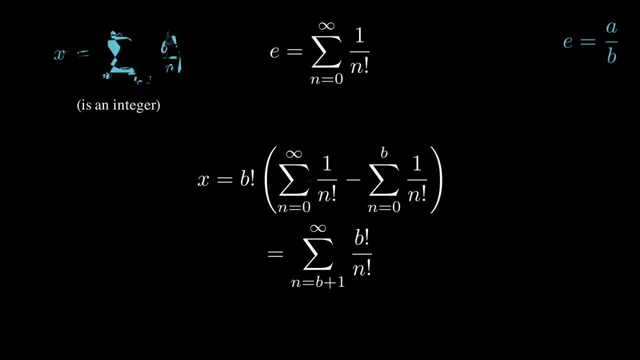 combine these sums, just summing from b plus 1 up to infinity, And the thing to notice here, all of the terms will be positive. In other words, our quantity x is strictly greater than 0.. Here comes the big reveal. If we write out this: 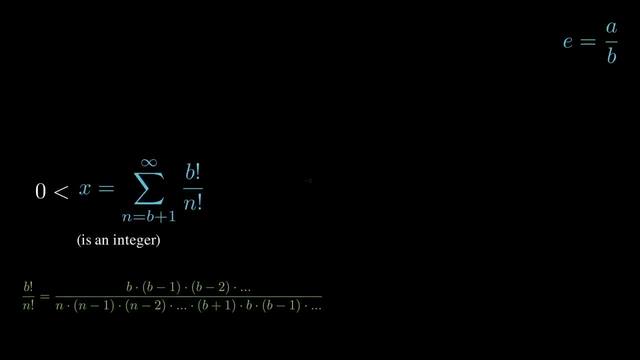 quantity. using the definition of factorials, we will see some canceling going on, since n inside our sum starts at b plus 1, in other words, n is greater than or equal to b plus 1.. What that means is everything in the numerator cancels out and we have this sort of truncated 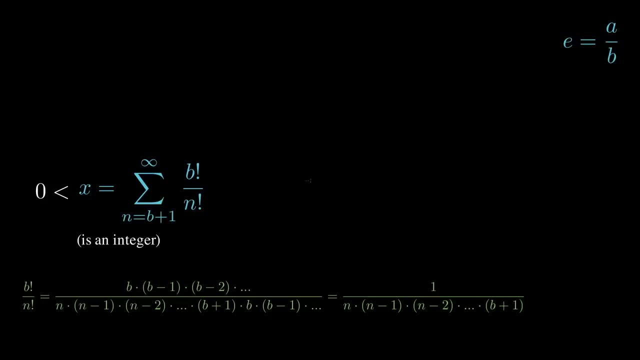 factorial of n down clean b plus one in the denominator. If you count those terms, we'll have n minus b of them, b plus one being the smallest term we can actually write a bound for this. this quantity is going to have to be less than or equal to if every term in that product was b plus one. 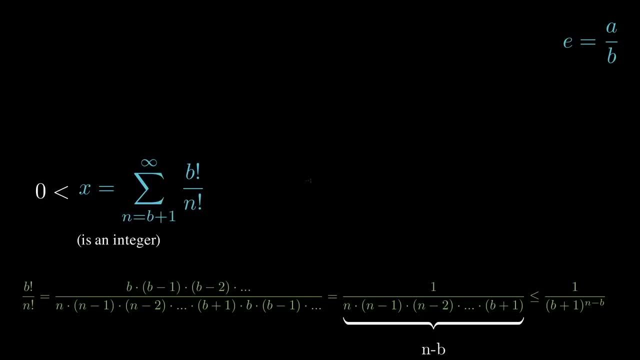 since b plus one is the smallest one. Here's the most fun part: We have this representation of this sum. Now we can re index it to make it look a little nicer like a geometric series. we know the sum of a geometric series, the first term divided by one minus the ratio. This simplifies. 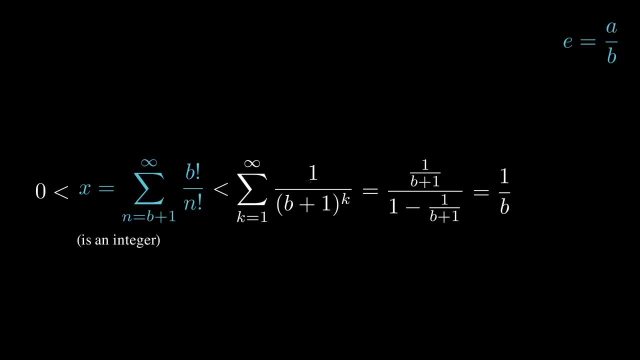 to one over B, Recalling that in our original assumption, B was a positive integer. one over B has to be strictly less than one. In other words, our quantity x, which is an integer, is greater than zero And less than one. There is no integer greater than zero and less than one. This is the